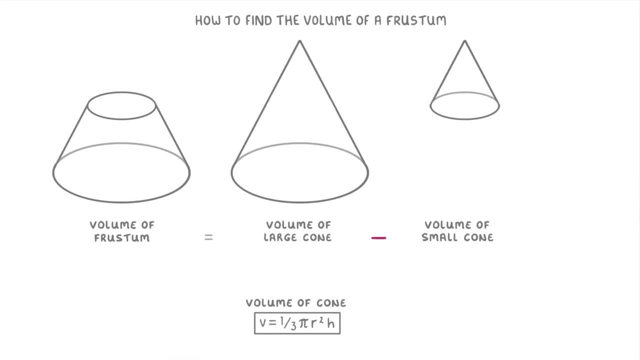 is 1 third pi r squared h. But to distinguish between the larger and smaller cones we often use uppercase R and H in the formula for the large cone and lowercase R and H in the formula for the smaller one To see this in practice. let's give it a try. 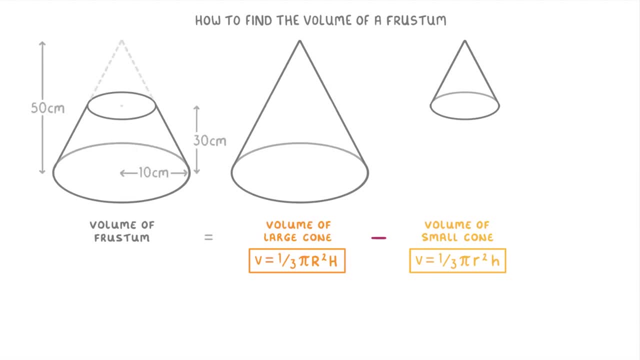 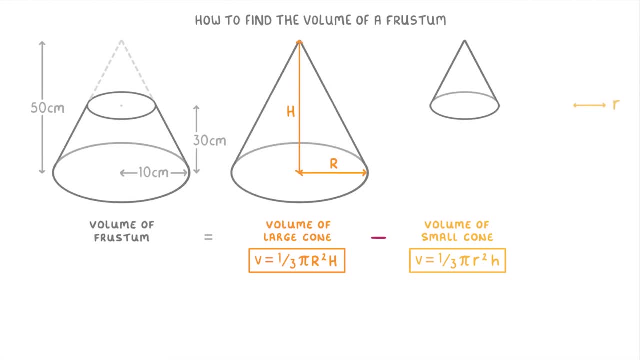 find are the radius and height of the large cone and the radius and height of the small cone. We can tell straight away that for the large cone the height is 50cm and the radius is 10cm because we were given those on our diagram of the frustum. 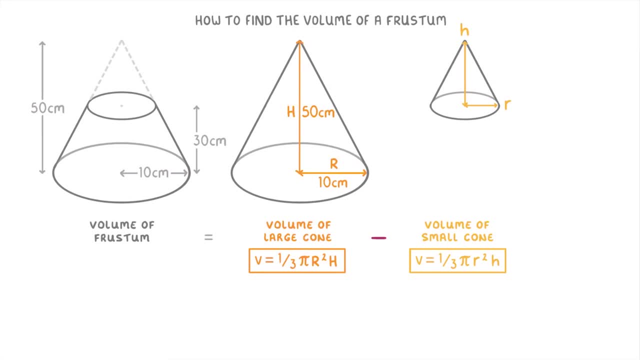 The small cone is a bit trickier, though, because we're not directly given its radius and radius or its height in our diagram. We can work out the height fairly easily, though, because it's just this distance here which must be the difference between 30cm and 50cm, so it must be 20cm. 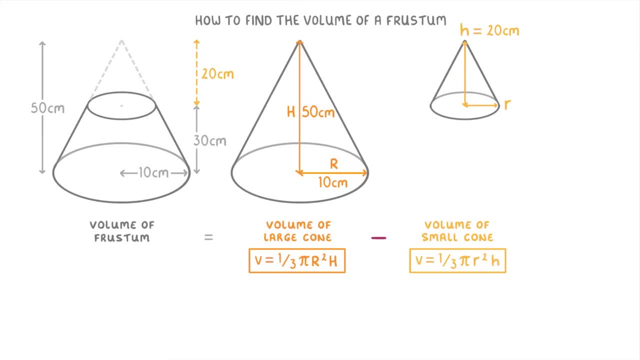 Now, to work out the radius of the small cone, we have to think of the large and small cones as similar shapes and find out the scale factor between them, Because if we know how many times smaller the small cone is than the larger one, we'll 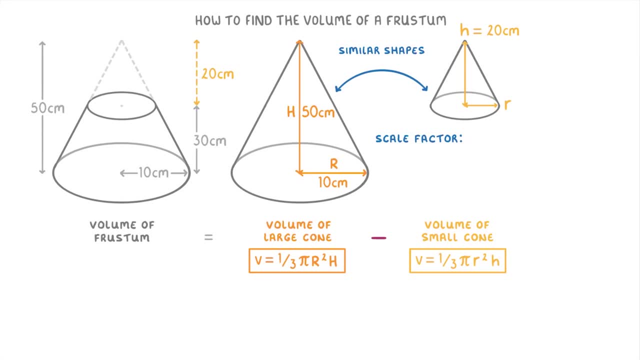 also know how many times smaller the radius is. To find the scale factor, we can do the large cone's height of 50cm divided by the small cone's height of 20cm, which gives us 2.5.. So we now know that the small cone is 2.5 times smaller than the large cone. 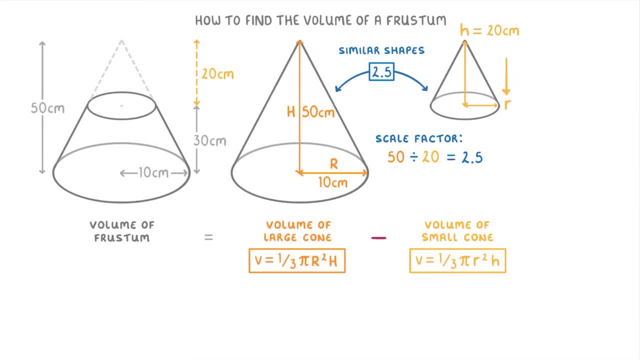 And so to work out the smaller cone's radius, we just do the radius of the big cone and the 10cm divided by the scale factor of 2.5, which gives us 4cm as the radius of the small cone. 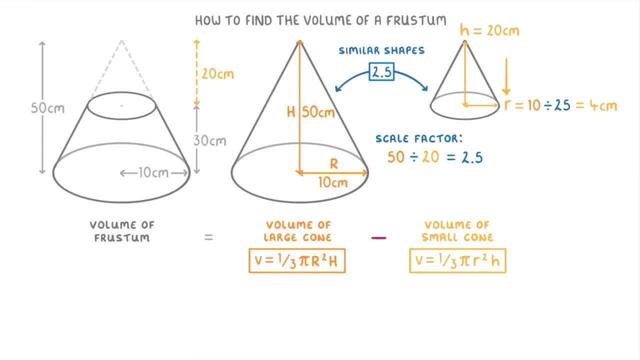 Okay, so we've now done the majority of the hard work, which is finding out our unknown radiuses and heights. Now all we have to do is plug them all into the formula. So the volume of the frustum is equal to the volume of the large cone, so 1 third times. 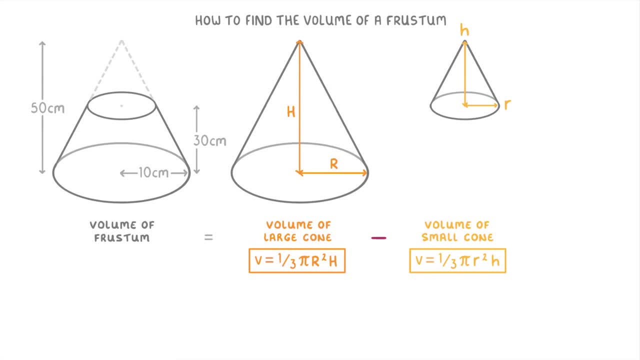 cone. We can tell straight away that for the large cone the height is 50cm and the radius is 10cm, because we were given those on our diagram of the frustum. The small cone is a bit trickier, though, because we're not directly given its radius and 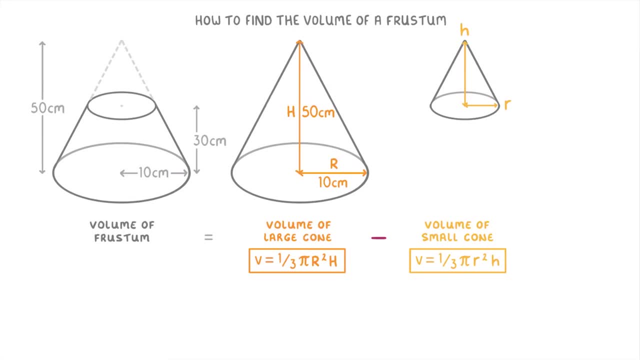 radius or its height. in our diagram We can work out the height fairly easily, though, because it's just this distance here which must be the difference between 30cm and 50cm, so it must be 20cm. Now, to work out the radius of the small cone, we have to think of the large and small cones. 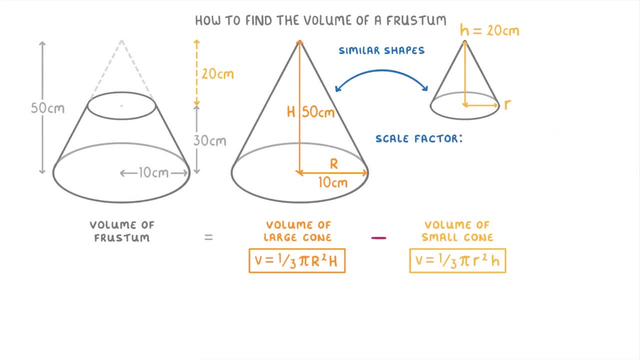 as similar shapes and find out the scale factor between them, Because if we know how many times smaller the small cone is than the larger one, we'll also know how many times smaller the radius is. To find the scale factor, we can do the large cone's height of 50cm divided by the small. 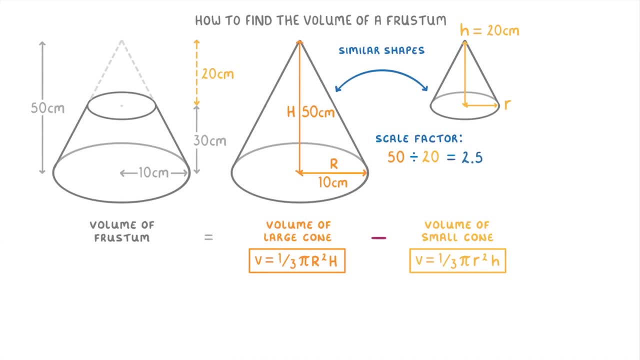 cone's height of 20cm, which gives us 2.5.. So we now know that the small cone is 2.5 times smaller than the large cone, And so to work out the smaller cone's radius, we just do the radius of the big cone and 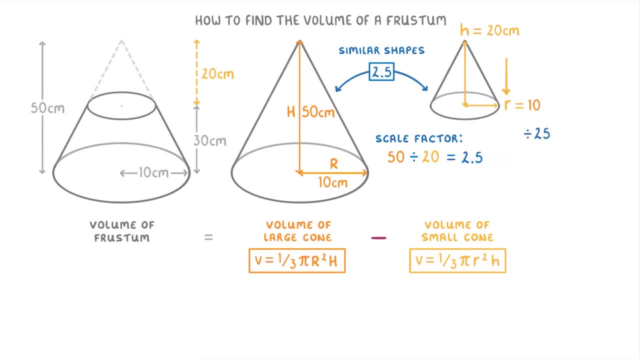 the 10cm divided by the scale factor of 2.5, which gives us 4cm as the radius of the small cone. Okay, so we've now done the majority of the hard work, which is finding out our unknown radiuses and heights. 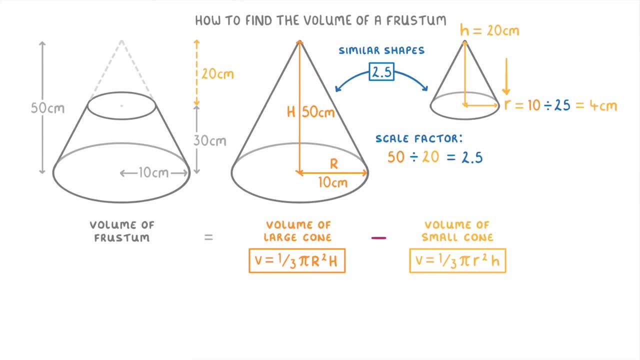 Now all we have to do is plug them all into the formula. So the volume of the frustum is equal to the volume of the large cone, so 1 third times pi times the radius of the small cone, So the volume of the frustum is equal to the volume of the large cone, so 1 third times. 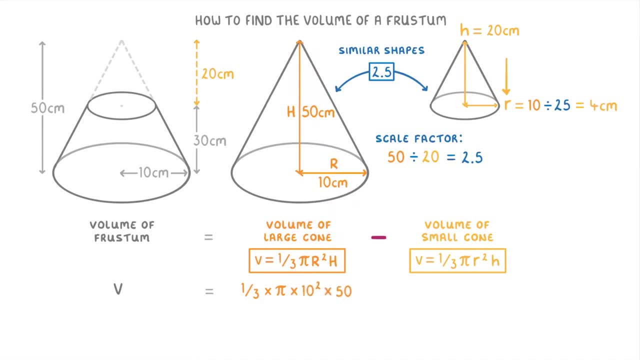 pi times the radius of 10 squared times the height of 50.. Take away the volume of the smaller cone, So 1 third times pi times the radius of 4 squared times the height of 20.. And if you're doing that by hand, that will simplify down to 5000 over 3pi minus 320. 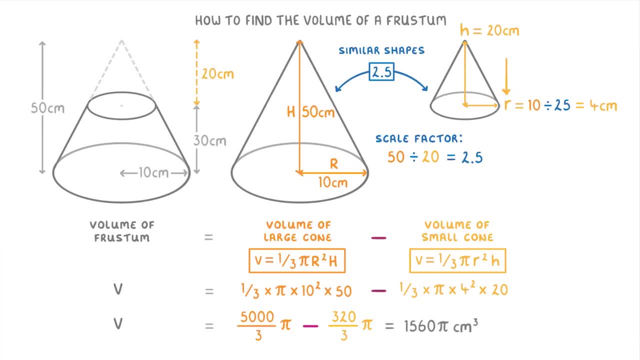 over 3pi. So our answer would be 1560pi centimetres cubed, Or, if you had a calculator, answer 1 to 2.. Answer 1 to 3.. Question 1 to 2.. Answer 1 and 3..